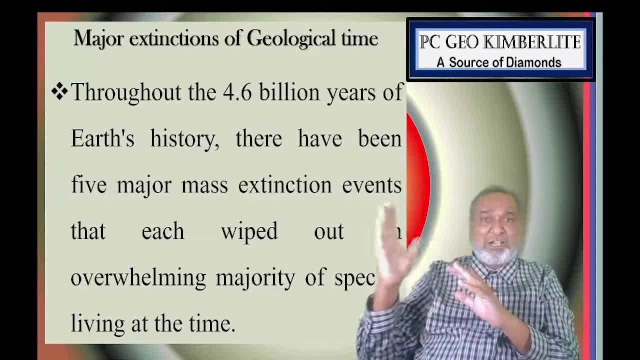 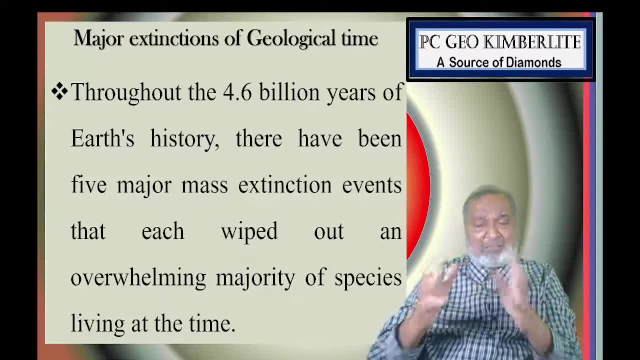 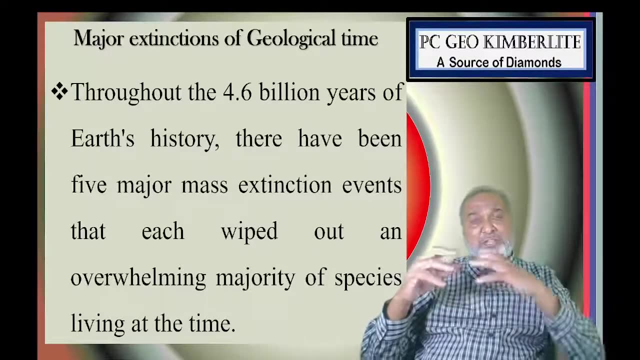 means 1000 million years. 1 million means 10 lakh. If you go on multiplying it is unimaginable. So here geologists who have the interest, they have to go on making whatever the geological events which have taken place in the past, in millions or billions years, he has to visualize. 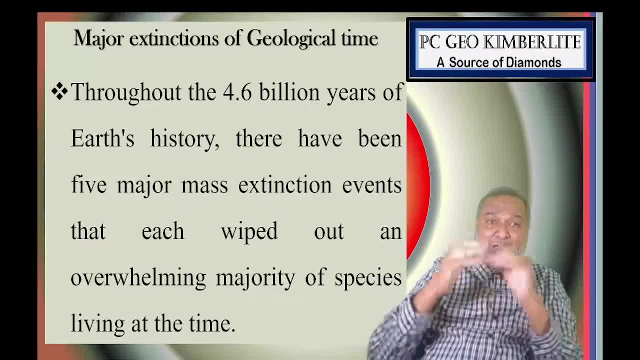 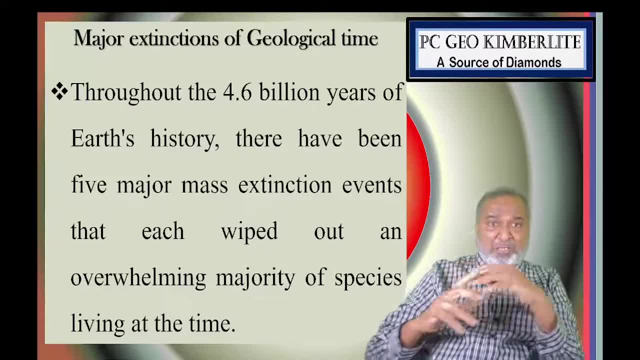 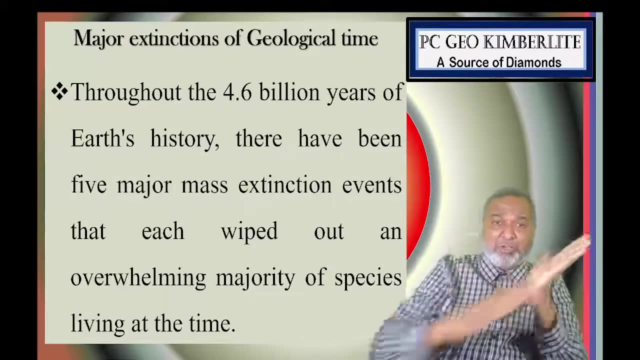 and he has to give his ideas based on whatever the documents he has got in the form of fossils or in the form of rock. So there has been five major mass extinction which has happened on the surface of the earth due to this Majority. which of the species which are living at that? 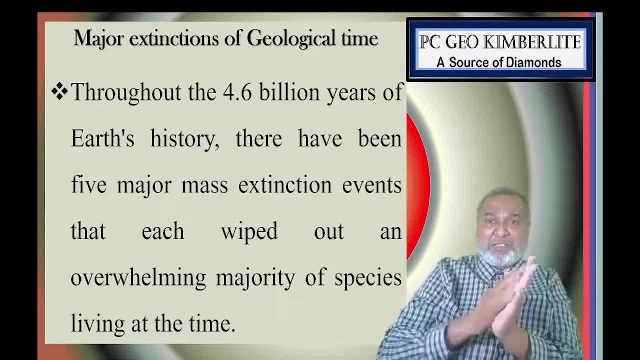 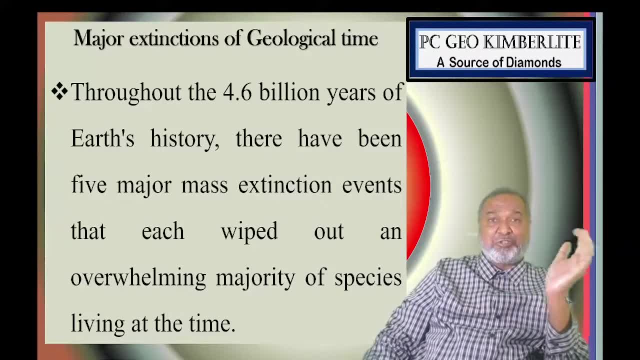 time. they have been gone. Whether it may be more than 50%, more than 75%, more than 96% of the species which are living in the earth, they have been gone. So there is no evidence of this particular, whatever the extinctions which are happening in that the 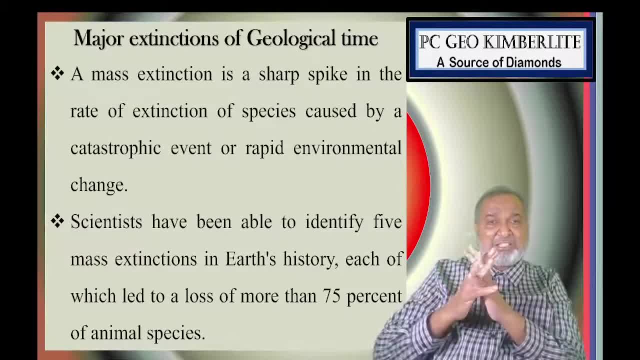 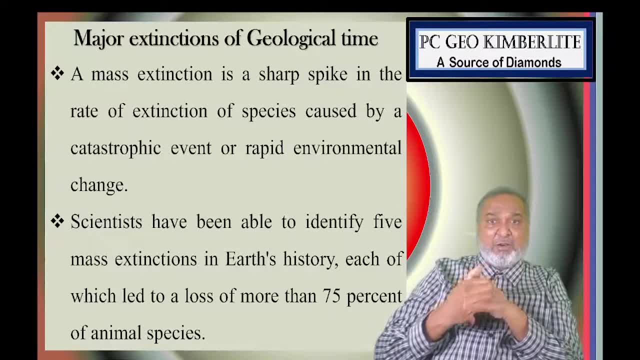 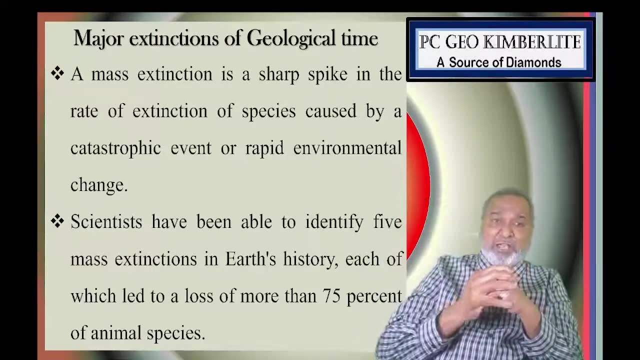 flora and fauna. they have been extinct. What is the mass extinction? It is a sparse pipe in the rate of extinction of the species caused by the catastrophic events or rapid environmental change. So these are the two important events. Catastrophic means which any unknown asteroids 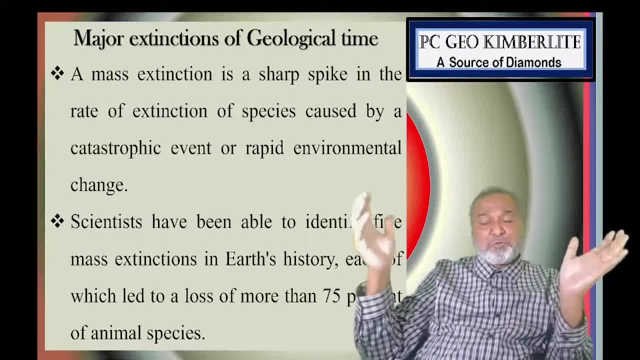 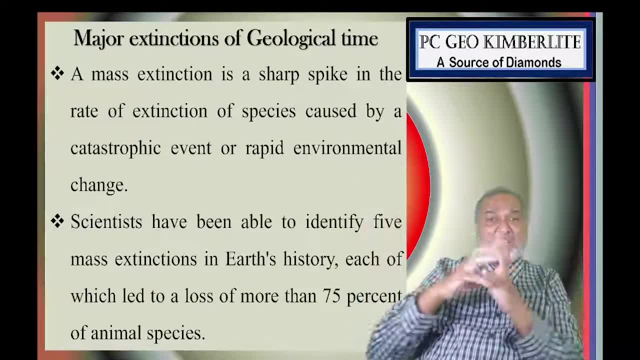 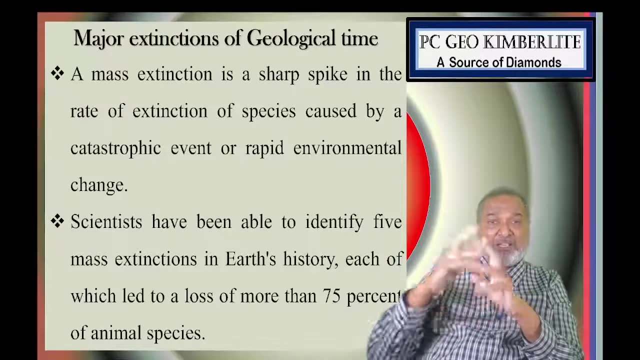 will have an impact on the surface of the earth and, due to that, there will be huge energy has been released. So that is one aspect, and the second one is rapid environmental change. So that is also a very, very important phenomenon which has taken place in the past. due to that, we have 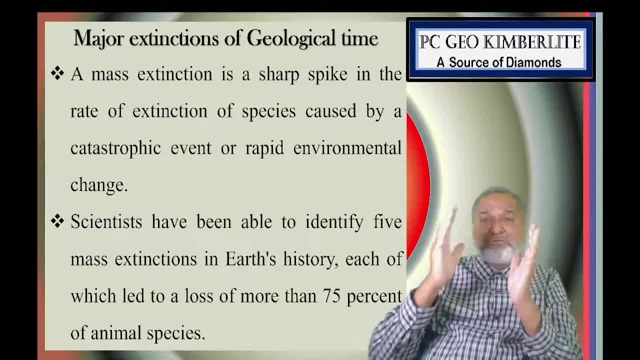 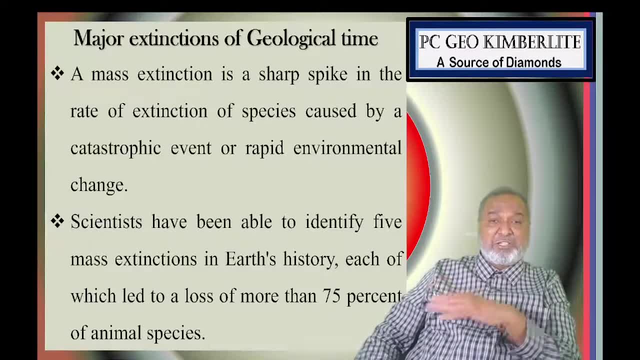 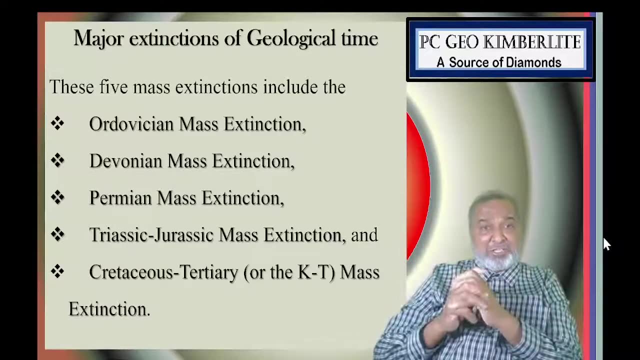 the five major extinctions. Scientists have identified five major mass extinctions in the earth's history. Each will lead down to a loss of major mass are the more than 75 percent of the animal species. and these are the five major mass extinctions. First one: Odovician mass extinction. Now we are going to see whatever the extinction. 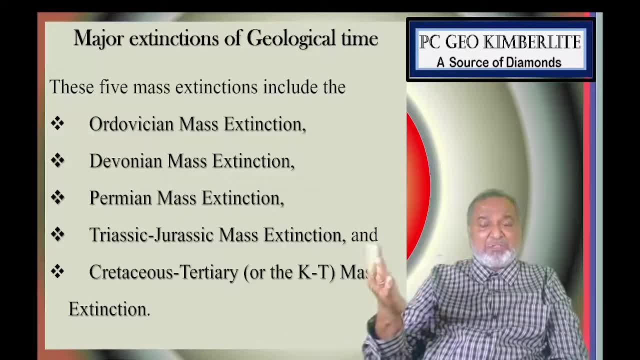 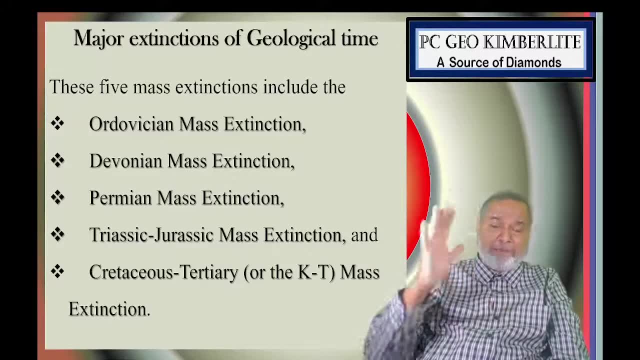 which are happening in the Paleozoic, because there will be the fossils which we are going to make, So Cambrian, Odovician, Silurian, Daonian, Carbonibense, Permian. This is the Paleozoic era is there and from that Paleozoic we are going to have three major mass extinctions. 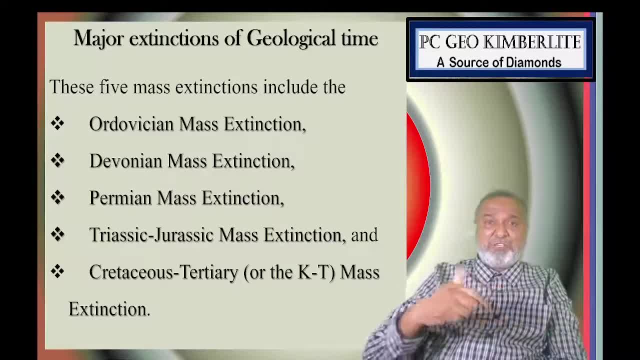 First one: Odovician mass extinction between Odovician and Silurian. Next one: immediately there is a Daonian is there and after the Daonian the next one is Permian mass extinction, Permian, Triassic mass extinction. That is the three major extinction which is happening. 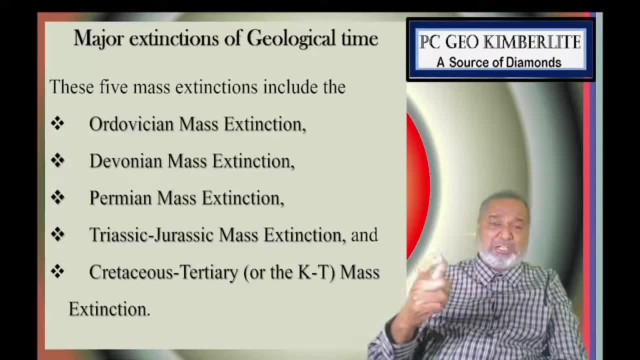 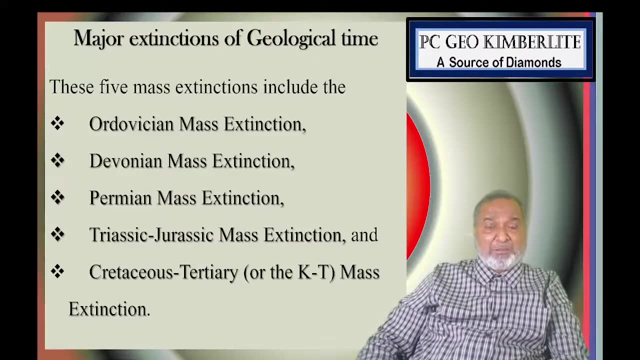 in the Paleozoic, whereas in the case of Mesozoic intermediate state, we have Triassic and Jurassic mass extinction and the next one is Cretaceous Tertiary mass extinction. So these are the five major mass extinctions which are happening on the surface of the earth, and each of these 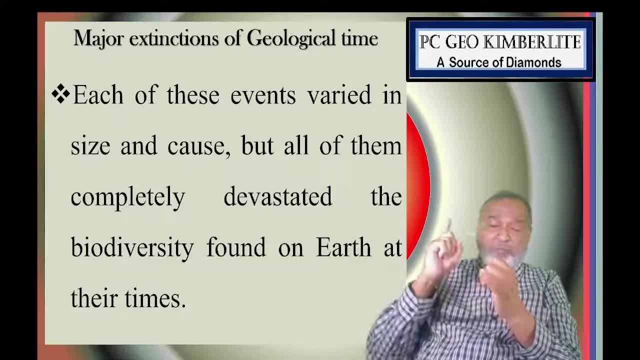 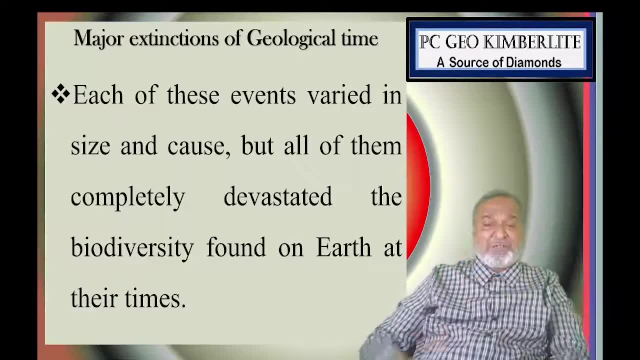 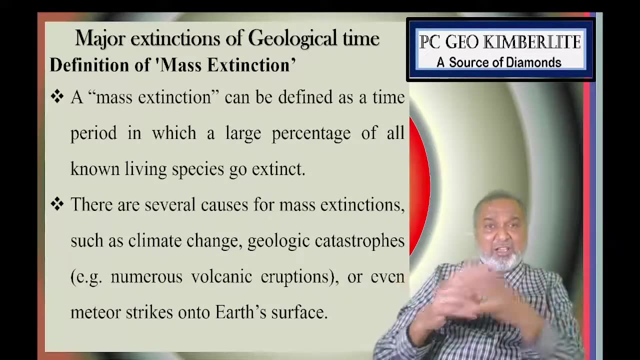 event which is varies in first their size, what will be the causes? but all of them completely devastate the biodiversity which is found on the surface of the earth at that particular time. So we will see first the simple definition of the mass extinction. Mass extinction can. 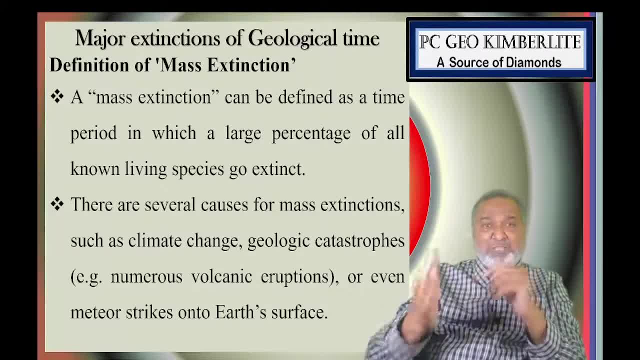 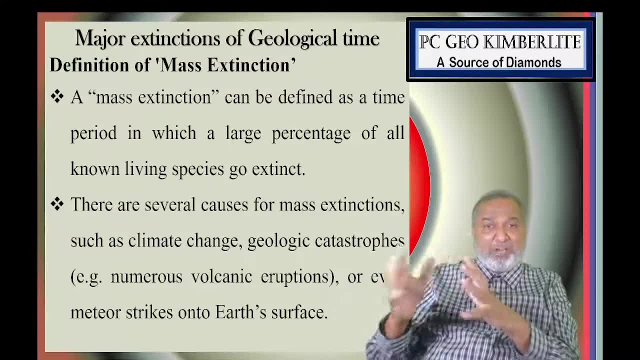 be defined as a time period in which a body is in a state of mass extinction, So the in which a large percentage of all known living species go extinct at one time. There has been several causes for mass extinction, such as climate change, geological catastrophes. 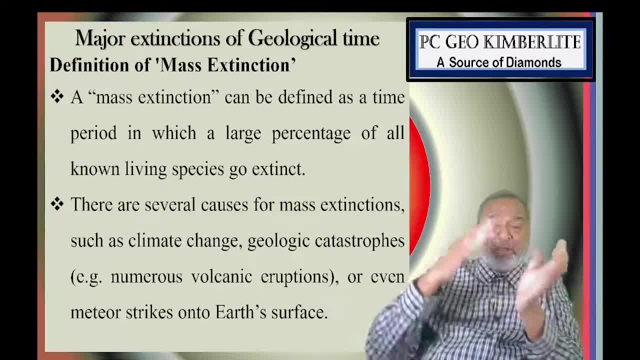 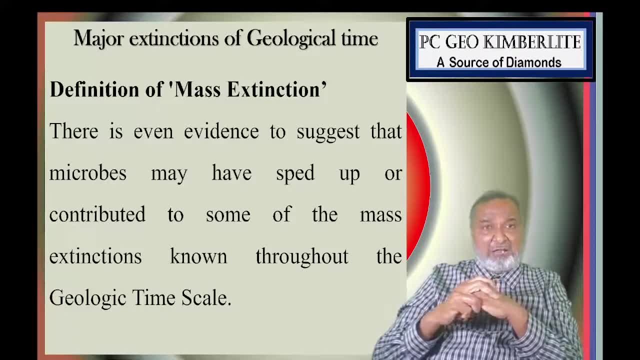 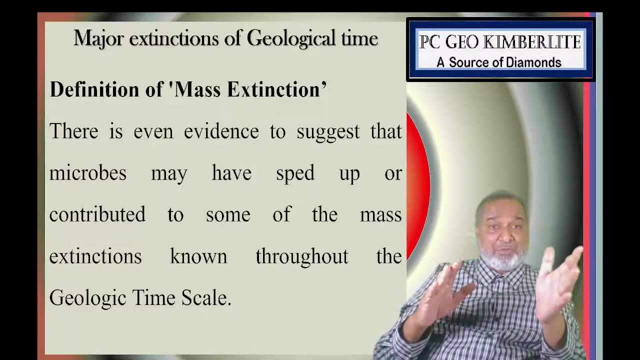 numerous volcanic eruptions which have taken place. even meteoroids strike on the surface of the earth. So these are the reasons which have been given by the various scientists at a various time for the whatever the five major extinction which is happening. There is even evidence to suggest that the microbes may have the spread up or contributed. 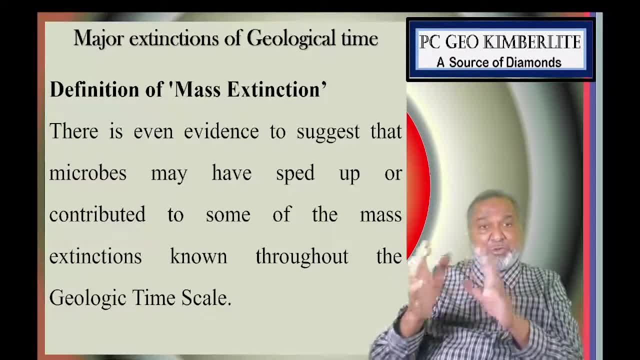 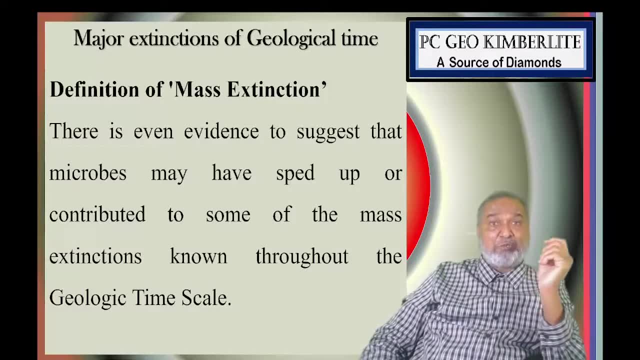 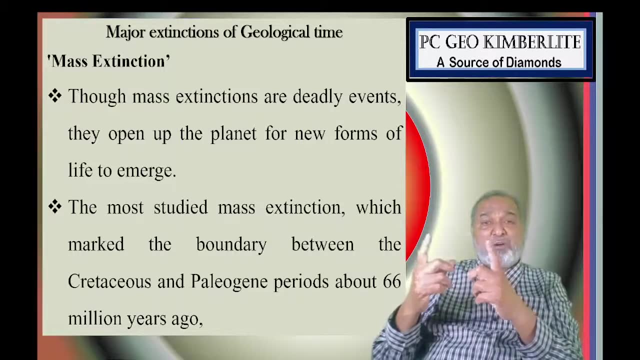 to some of the mass extinction known throughout the geological cycle. So they have been playing a vital role in converting the climate change. the microbes also play a vital role. Though the mass extinction was a deadly event, they open up the planet for new form of life. 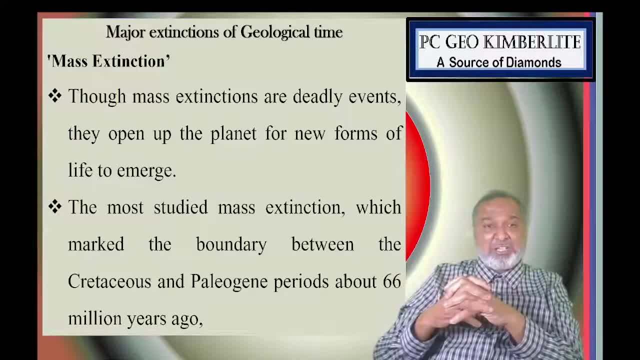 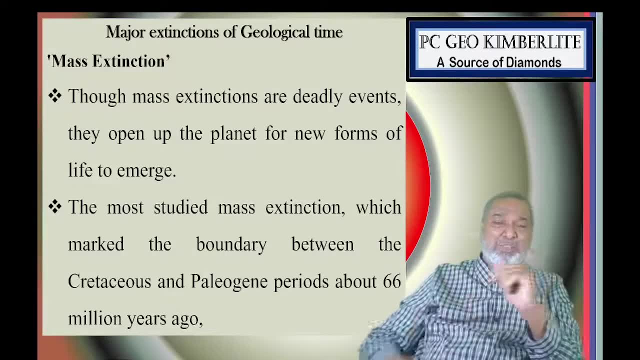 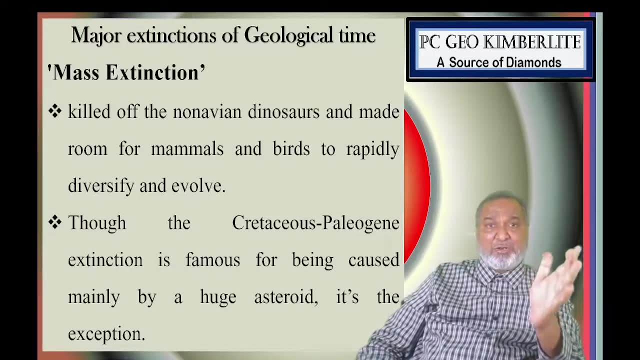 to emerge. the most studied mass extinction, marked by the boundary between the Cretaceous and Pelagian period, that is, about 66 million years ago back, that is the K-T boundary, Killed off the non-avian dinosaurs and made room for the mammals and birds to rapidly diversify and evolve. Though the Cretaceous Pelagian 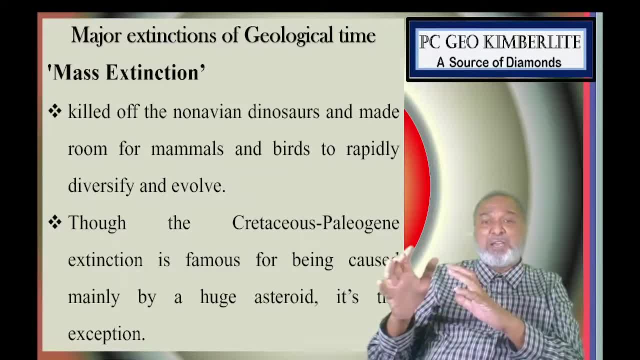 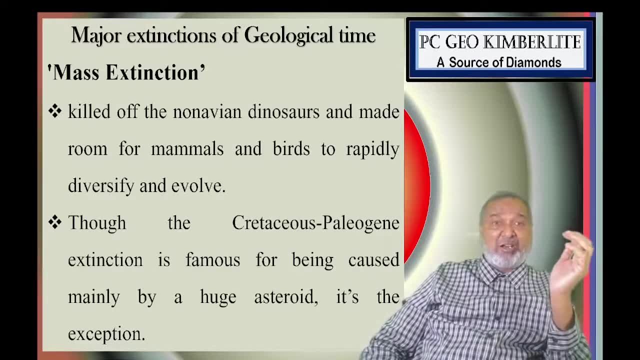 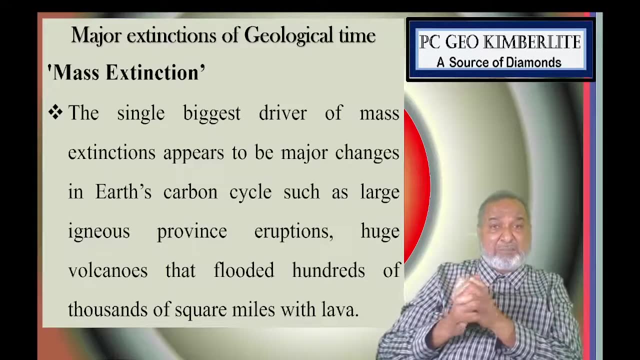 extinction is famous for being caused mainly by huge asteroid is going to hit the surface of the earth, So that is the major reason for the mass extinction of the K-T boundary. The single biggest driver of the mass extinction happened to be the major changes in the earth's 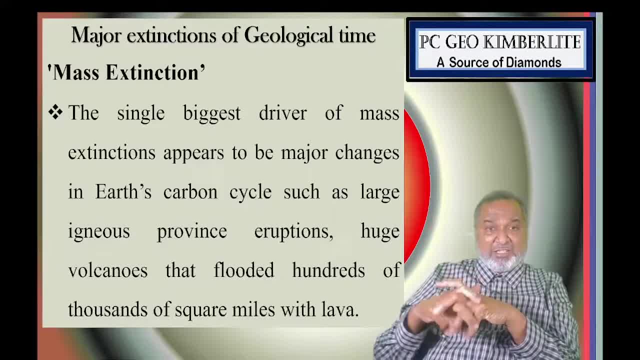 carbon cycle. that is also a very, very important reason, such as large igneous prominence, is eruption, Like what we have is the eruption of the Cretaceous Pelagian period. So the Yellowstone Park, the volcanic eruption which has taken place, that is a huge gases magma. 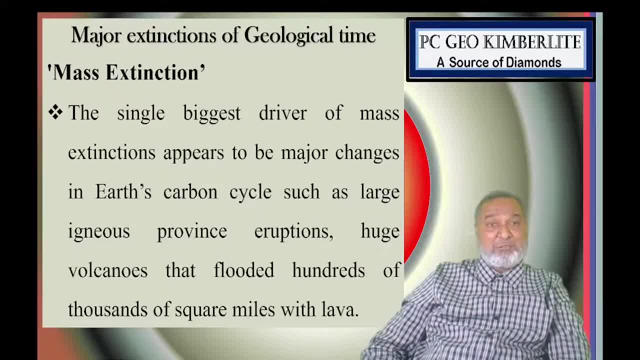 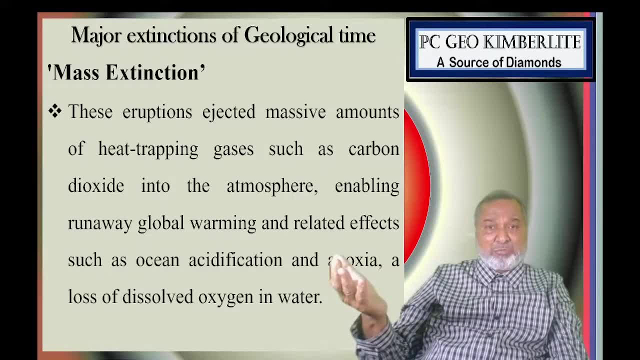 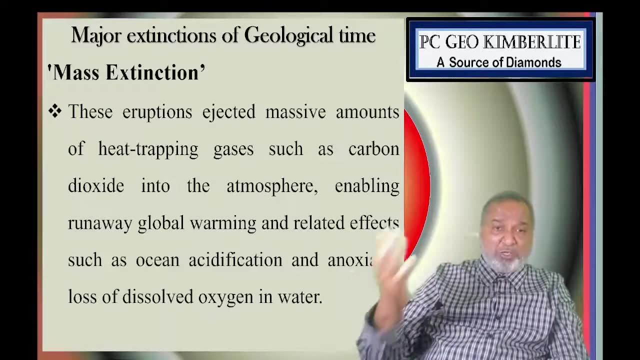 has been poured on the surface, thousand square kilometer, which has been spread up with the lava. These eruptions ejected a massive amount of heating trapping gases such as carbon dioxide into the atmosphere, enabling a runway, global warming and related effects such as ocean acidification, anoxia, a loss of dissolved oxygen in the water. So so many, the one by 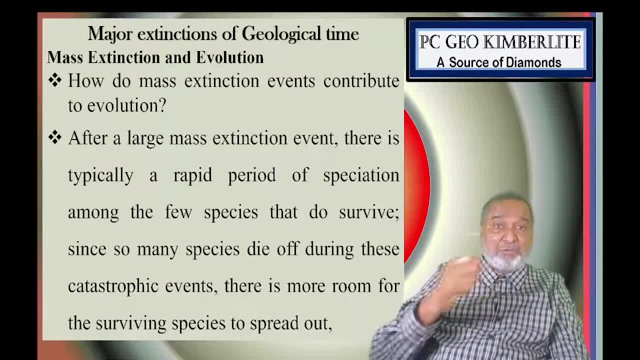 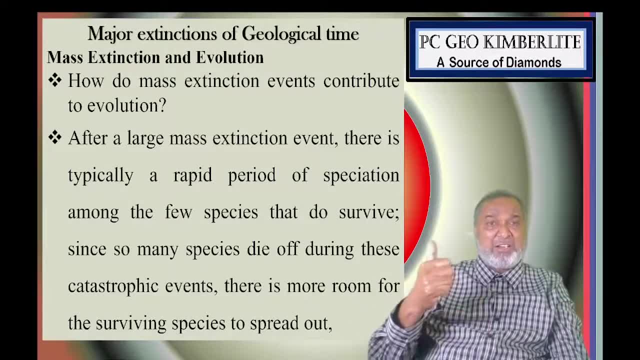 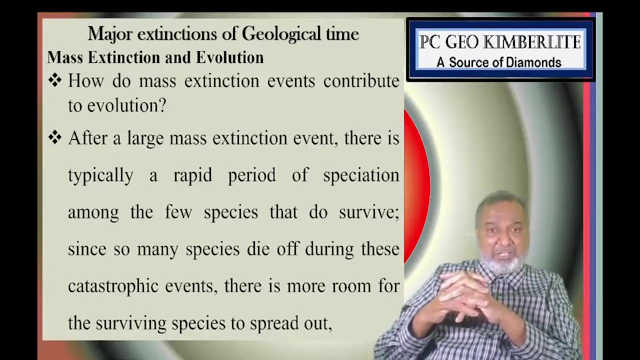 one. They are interlinked phenomena. Can we ask: how do the mass extinction event contribute to the evolution? After a large mass extinction event there is typically a rapid period of speciation among the few spaces that to be survived. So those who are the fittest to 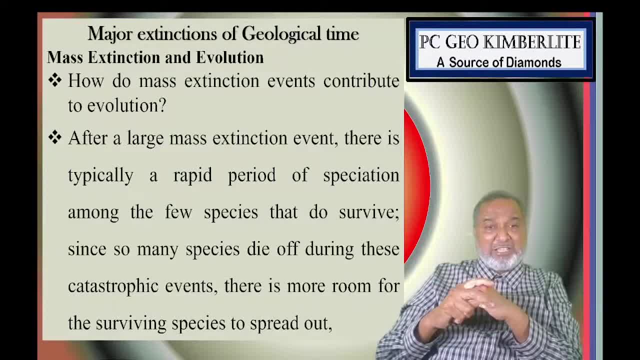 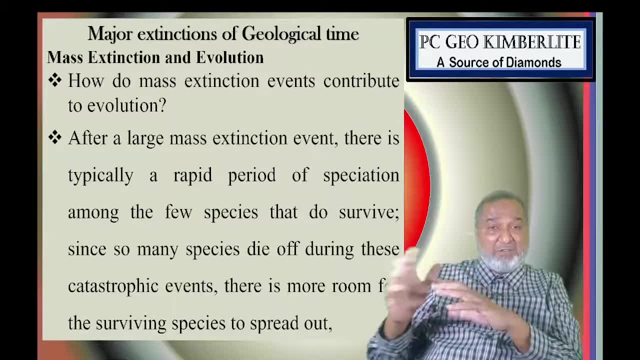 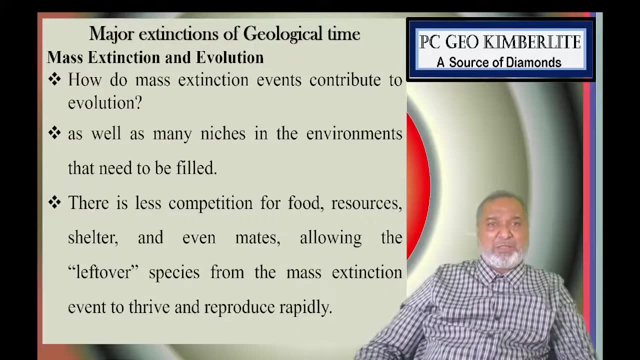 that particular extinction they will be survived. Since so many spaces die off during these catastrophic events, there is more room for evolution, So they will be there in that particular year as many as natures in the environment. that needs to be fulfill. There is a loss nest, competition for good resources, shelter, even meds allowing 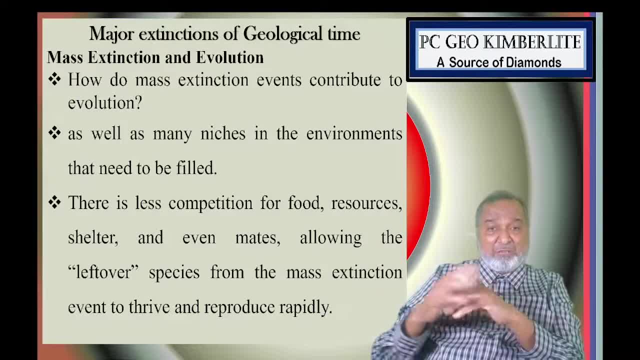 leftover spaces or the from the mass extension event to few and reproduce rapidly. Of course, they will be there in the future When we go against that efficient management. Also mats And it should be moistly humid When you're having food or any of these main cruise ships. 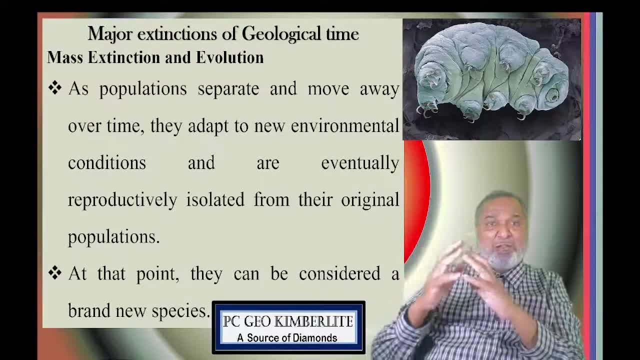 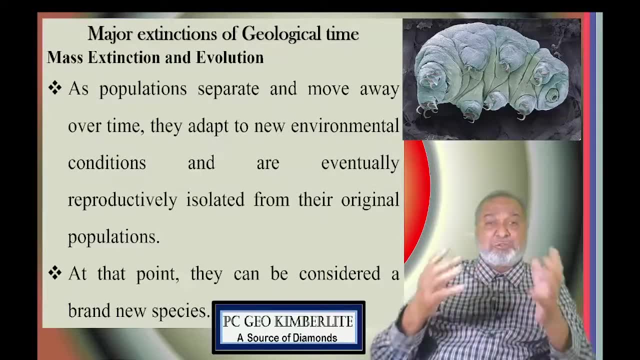 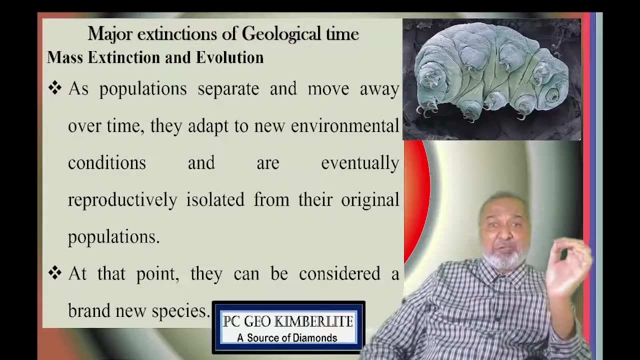 and they choose to call out to yourself, shouldn't it? I just arranged a short China traction survey. You're going to fall ahead thousand feet and ban them? The first demand and answer is: for one third Population separate more and more away from over the time. they adopt a new environmental condition and are eventually producing the isolated from their original population At that point can be considered as a brand new species will going to form on the surface of the earth. We will see, one by one, all the five major extinction. 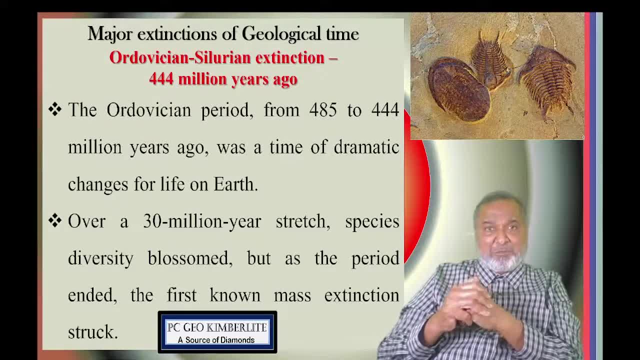 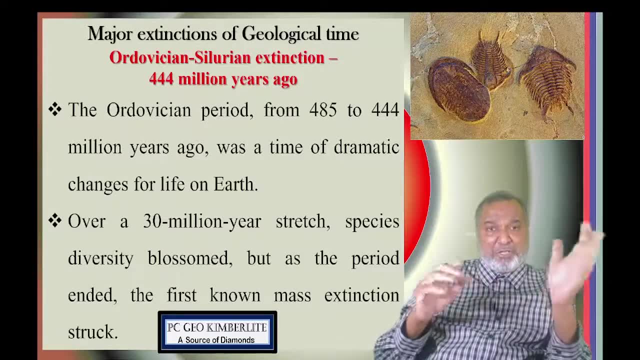 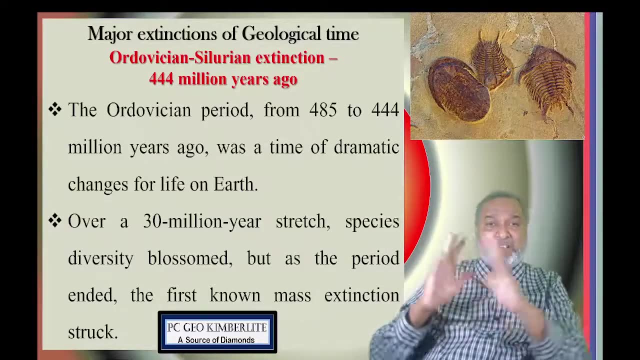 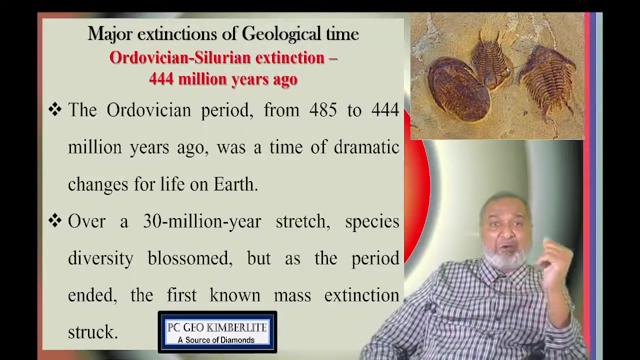 The first one, Ordovician Silurian extinction. It has been taken place way back, if you see, 444 million years back. So Ordovician period will be there from 485 million years to 444 million. That means 41 million year will be the total duration of the Ordovician period. That was a time of dramatic changes for the life on the earth. This is the first time. 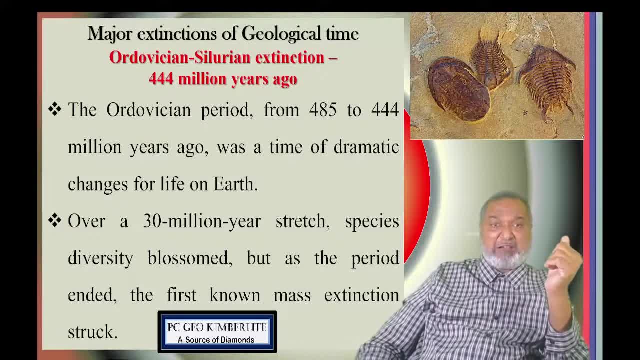 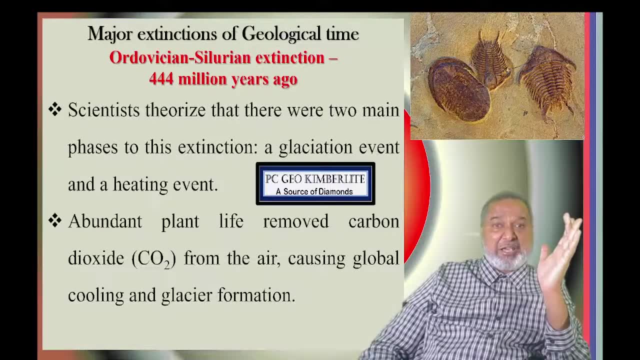 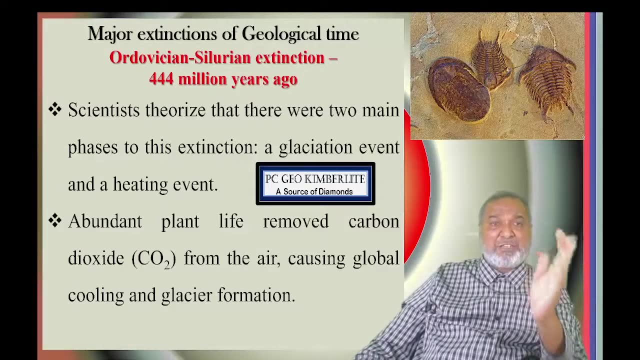 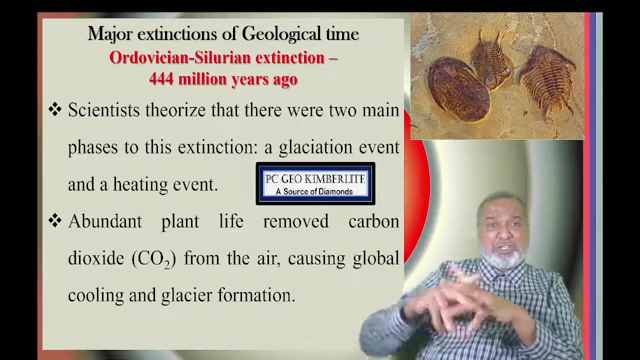 Over the 30 million years will be stretched. It will classify bloom. But as the period is going to end, the first known mass extinction will be extinct. And scientists, there are theories that there were two main phases to be this extinction. One is glaciation event and a heating. First there is a glaciation and after that there is a heating event. 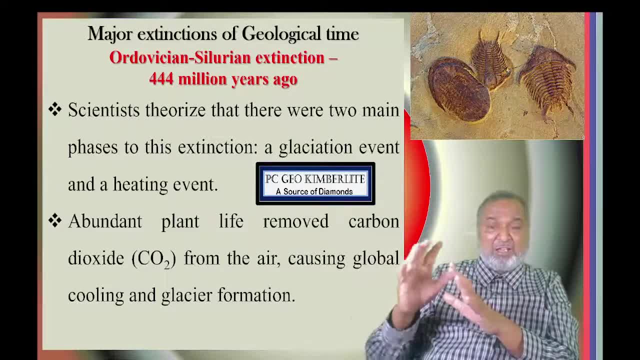 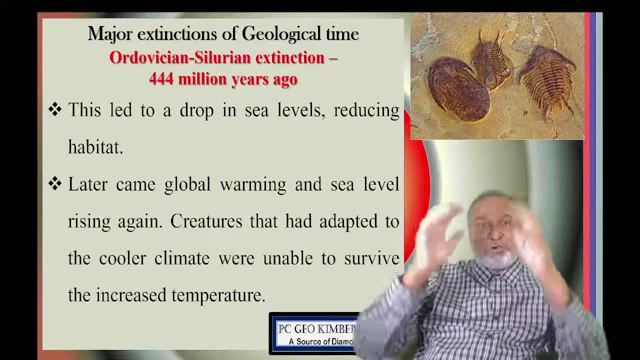 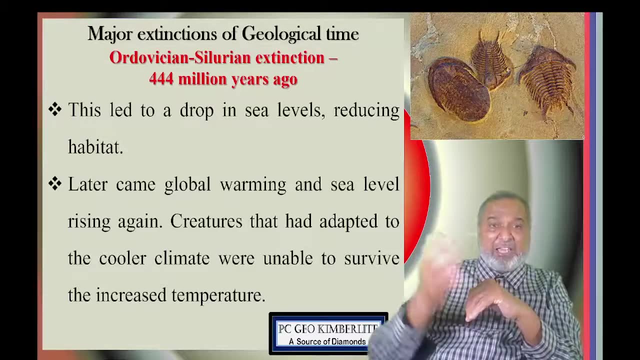 Abundant plant life removed carbon dioxide from the air, causing global cooling and global warming. Second, there is a massive glaciation formation that leads to the drop in the sea level and reducing the habitat. Later came global warming, sea level rising again and creatures that had adapted to this particular cooler planet were unable to survive the increased temperature. 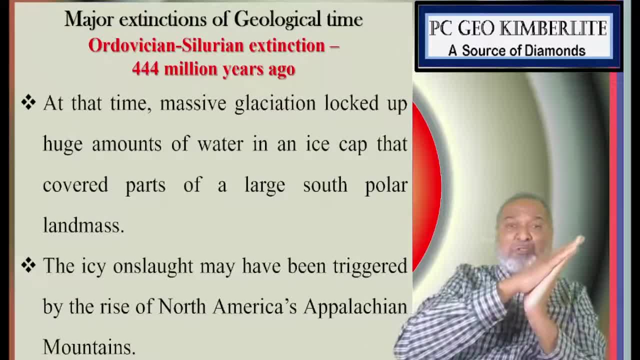 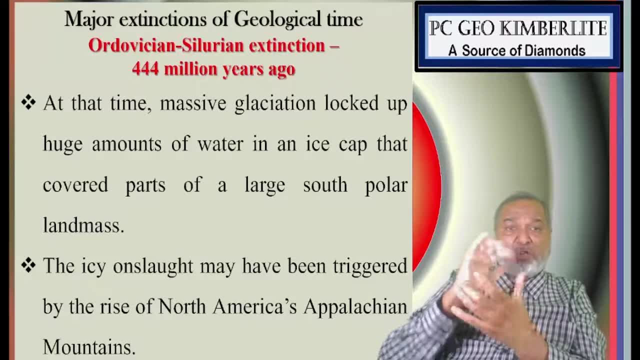 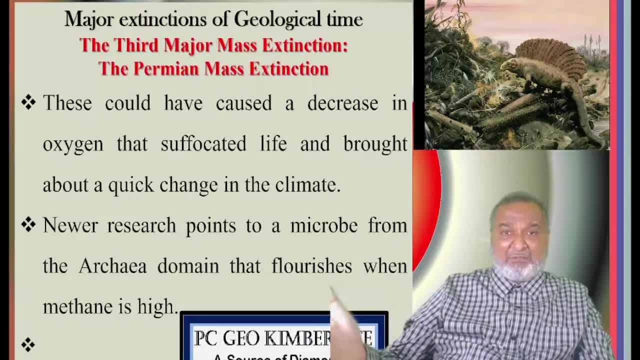 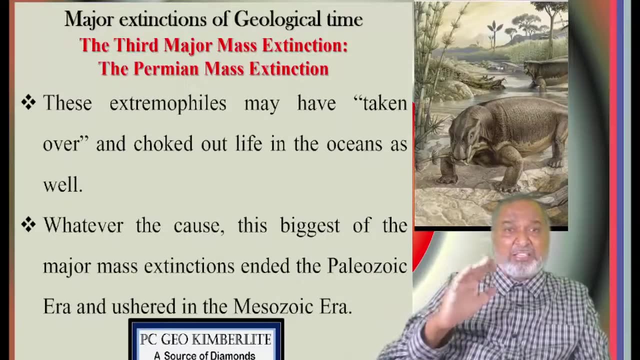 cause a decrease in oxygen that suffocated the life and brought about a quick change in the climate. newer research points to a microbe from the archaea domain that flourishes when the methane is high. these extremophiles may have taken over and chalk out the life in the oceans as well. 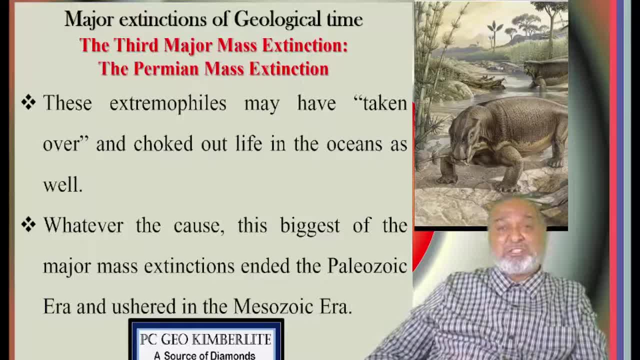 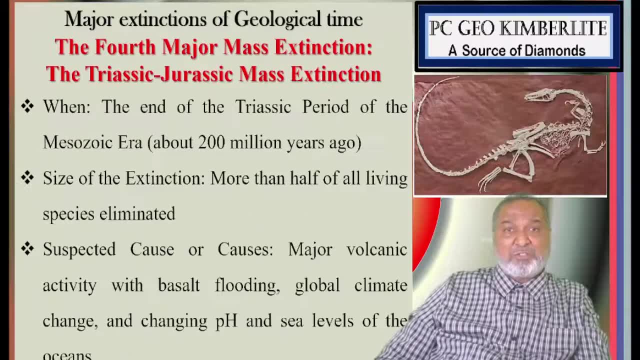 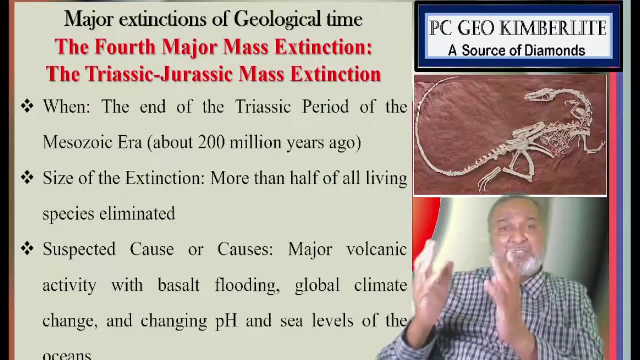 whatever the cause, this is the biggest of the major mass extinction ended in the ended the paleozoic era and you shall the in the mesozoic era. now come to the next one, the fourth major mass extinction, that is, the triassic jurassic mass extinction, where we have uh seen the so many 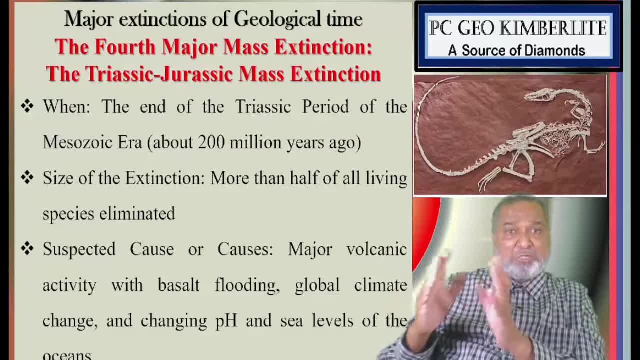 things, that is, the the end of the triassic period of the mesozoic era, that is, about 200 million years from now ago. the size of this extinction: more than half of the living spaces are eliminated. what are the causes? major volcanic activity with the basaltic flooding. global climate change, changing ph. 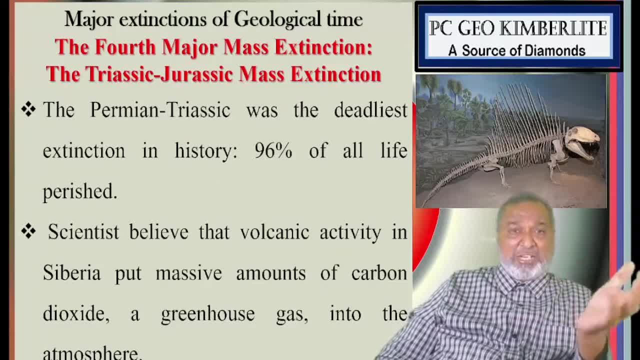 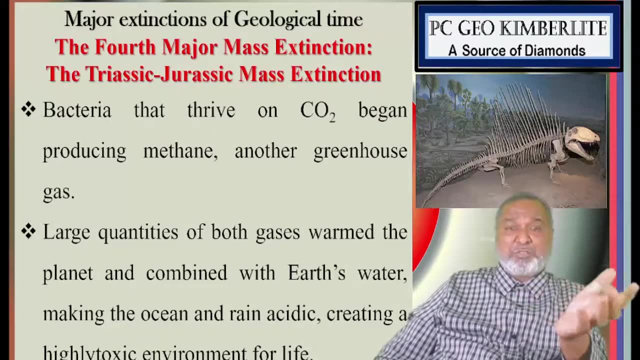 and sea level of the oceans. the permian triassic was deadiest, even in the attention: 96 percent has been dead. the scientists believe the volcanic activity in siberia put massive amount of the carbon dioxide as a greenhouse into the atmosphere and bacteria that drive co2 begin producing. 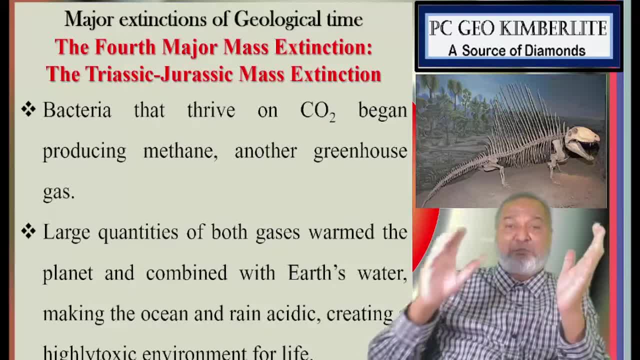 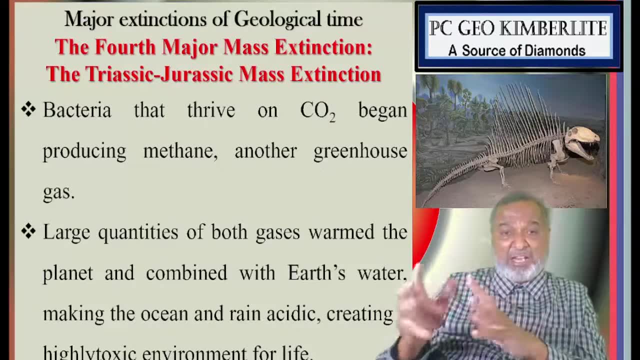 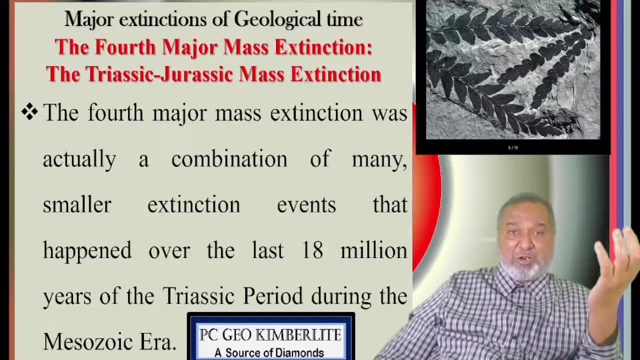 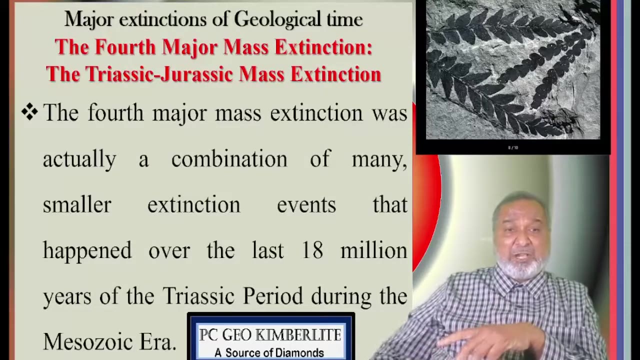 methane, another greenhouse gas, large quantities of both gases that what is called the basaltic acid acidity, and this acidity is created by theən 통 of the planet and combine earth's water, making the ocean and rain acidity, creating a highly toxic environment for the life. the fourth major mass action, actually a combination of the event that has happened. 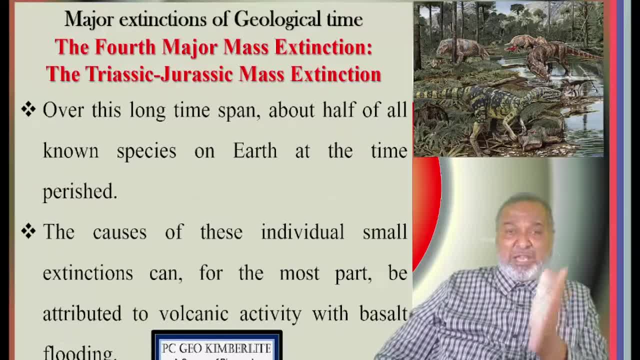 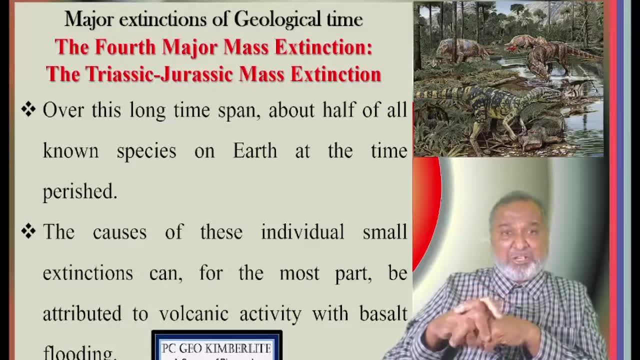 a last 18 million years of the triassic period during the mesozoic era for a long time span, half at that time is clearish Causes. of these individual small extinction can for the most part be attributed to the volcanic activity with the basalt flooding. 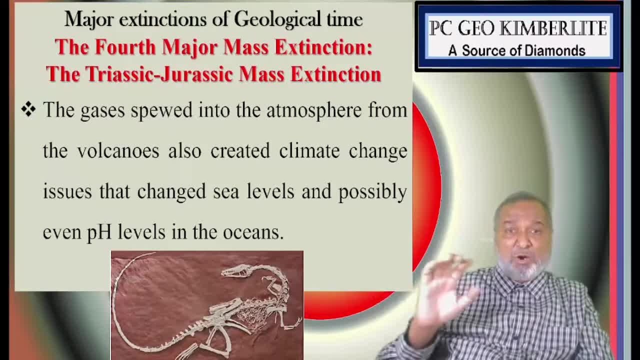 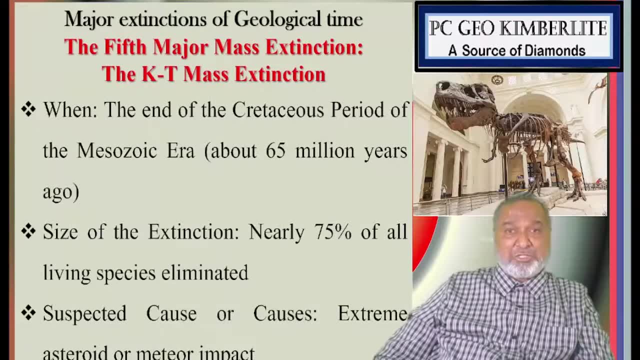 As a spew into the atmosphere from the volcanoes also created climate change issues that changed sea level, possibly even pH level in the oceans. The next one, the fifth major mass extinction that is called as the KT boundary Cretaceous and tertiaryThe end of the Cretaceous period, the Mesozoic era that is. 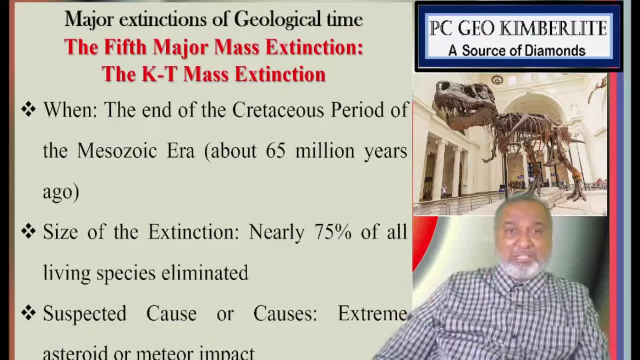 about 65 million years ago. The sites will be. nearly 75% of the living species are eliminated and there is extreme a asteroids or meteoroid impact. Climate change has given. many thing has been given here, but the still it is a debatable there, The. 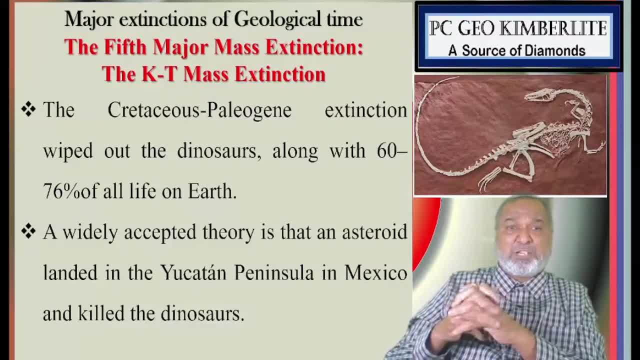 Cretaceous pearugenue extinction wipe off all the dinosaurs along with same water- separating new ones: 60 to 76% of the life on the earth. A widely accepted theory is that asteroid is landed on the Lucatan Peninsula in Mexico and killed the dinosaurs. The impact could have ejected 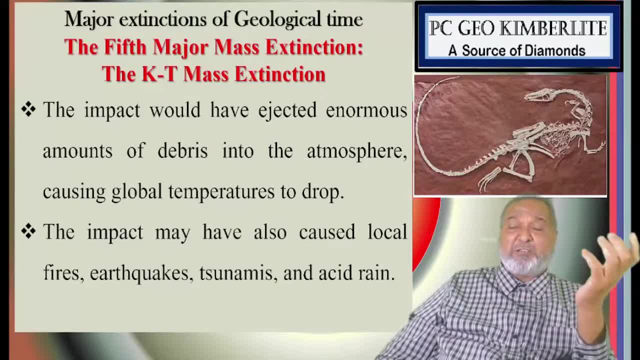 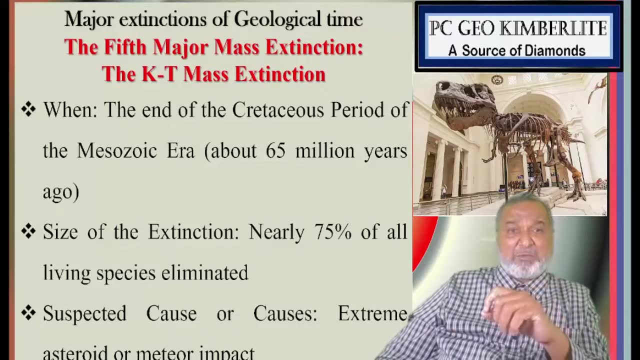 enormous amount of debris into the atmosphere, causing global temperature to be dropped. The impact may have also produced cause a local fires, earthquake, tsunamis and acid rain. End of the Cretaceous period of Mesozoic era. ie, 65 million years. size is about 75%. 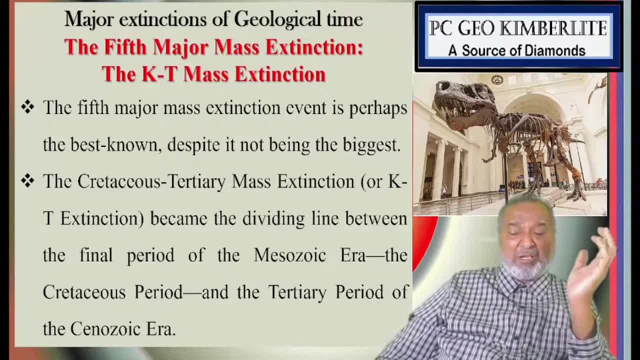 and suspected. that is a we have been talked about. that particular metroid or the climate change will be there. Cretaceous-tertiary boundary, ie dividing between the final period of Mesozoic era and the Cretaceous period and the tertiary of the Cenozoic. It is also 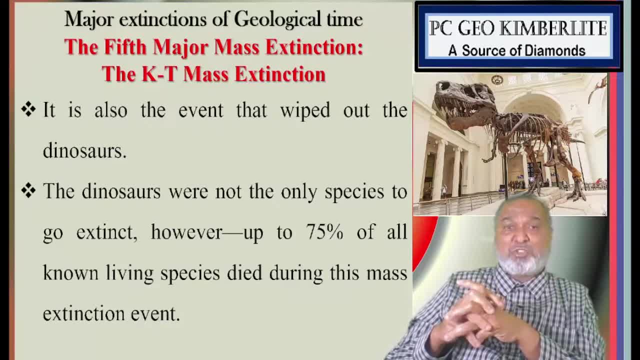 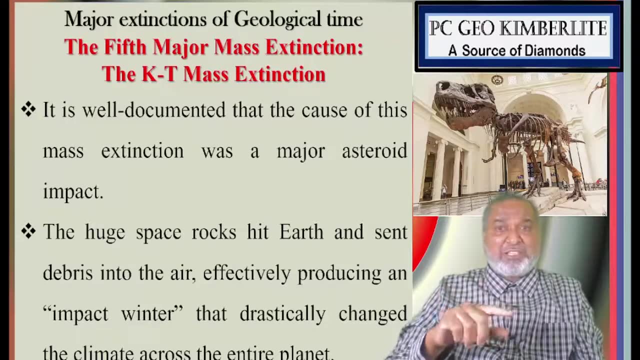 the event that wipe out the dinosaurs. The dinosaurs were not the only species that were there to go extinct, However. upto 75% of the known living species died during the mass extinction event. As well documented that cause of these mass extinction was a. 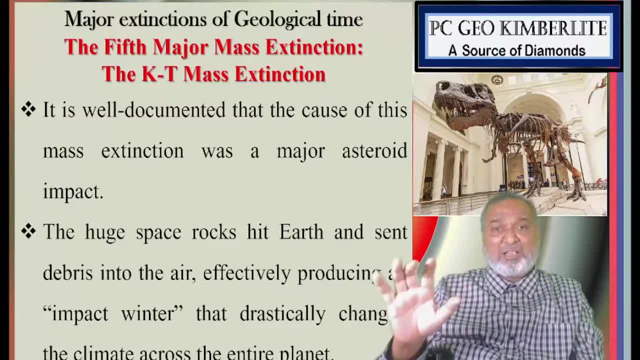 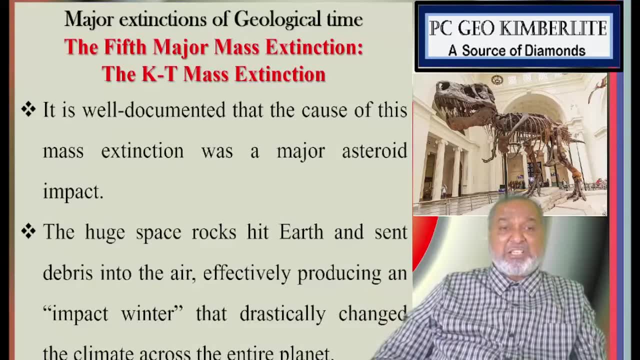 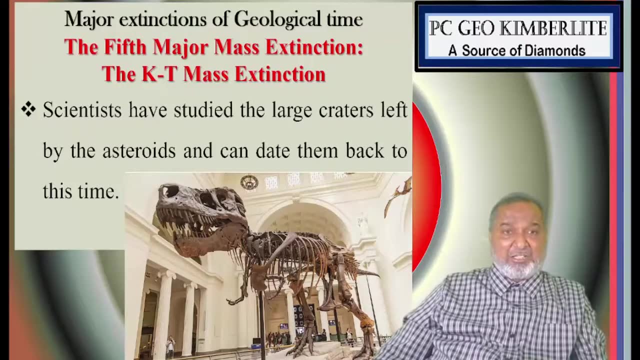 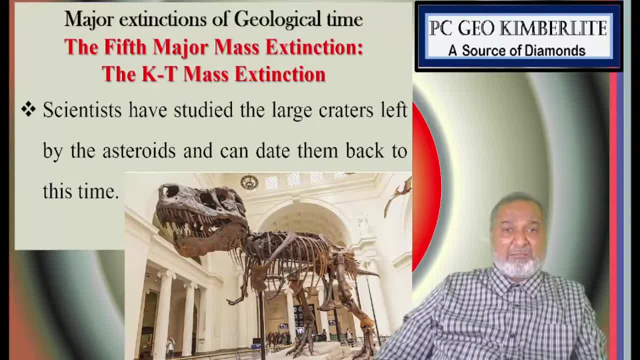 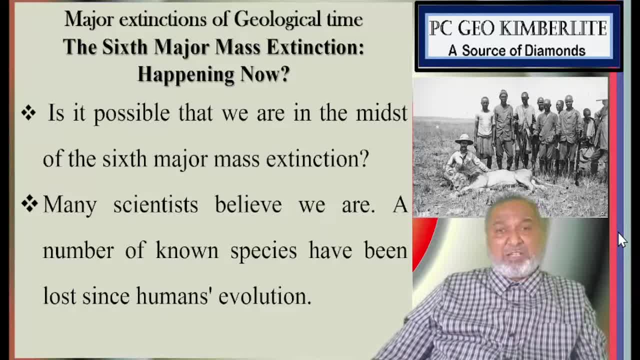 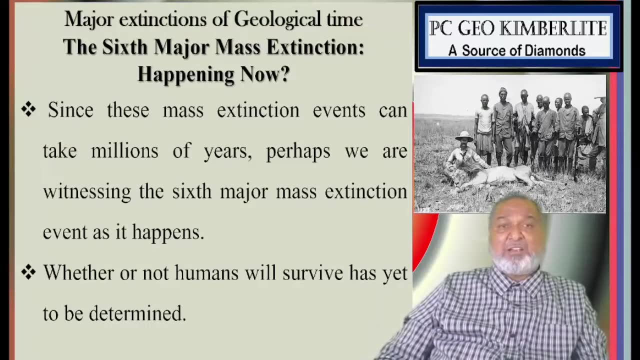 It is possible that we are in the middle of six major mass extinction. Many scientists believe we are. a number of scientific known spaces have been lost since the human evolution. Since these mass extinction events can take million years. perhaps we are witnessing the six major extinction event as it happens. 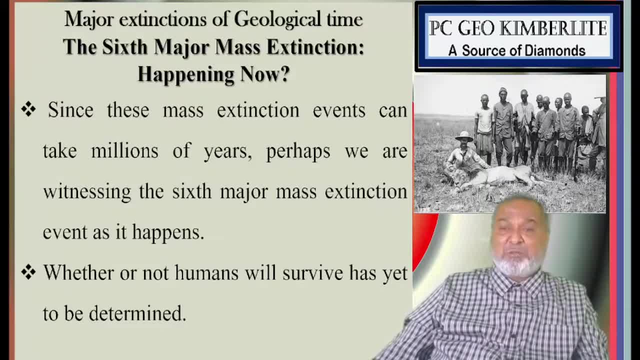 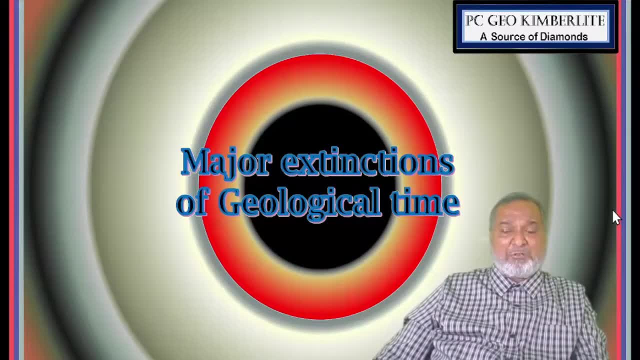 Whether or not a human will survive has yet not been determined. So what will be the future? We don't know. But these are the five major mass extinctions which are happen on the surface and six one we are going to witness. But whether we will be there in the after the survive or not, that is the question able. 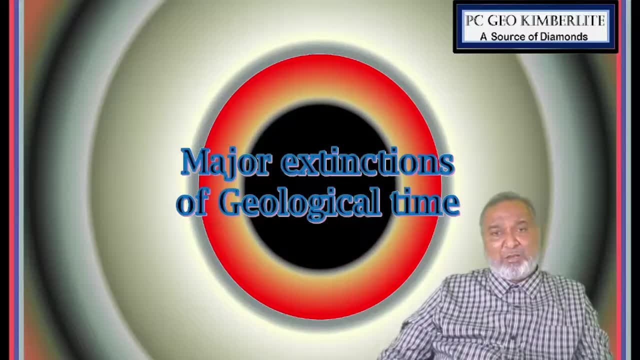 So if we have any questions, please write on the comment section so that I can give you the answers. Thank you, Have a nice day. Those who want to see the other videos of the pedagogy: stratigraphy: structural geology: 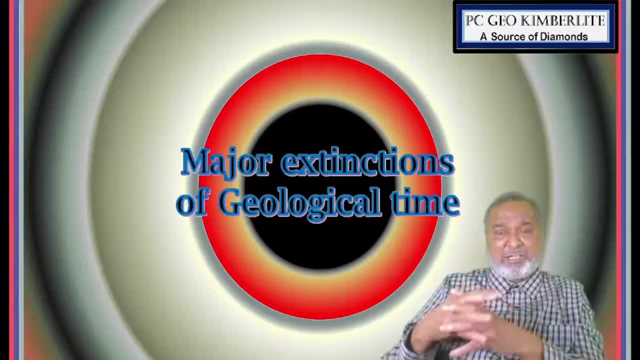 then crystallography, mineralogy and the practical basic practicals of the FIBSE. they can visit to my channel See that there are a number of folders have been made. In addition, the scholarship, national scholarships for all categories, minority- is there then. 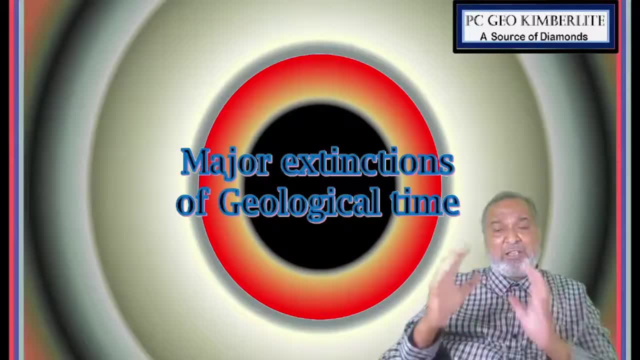 the open category, only the two criteria: the income limit and your academic record. Only these two- those who are there, that is called as the CSR scholarships- are there. They can go and watch, as per your requirement. Thank you, Have a nice day. Bye, bye.